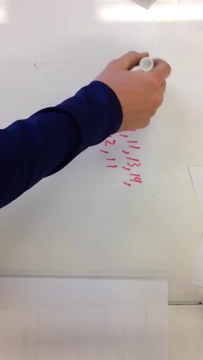 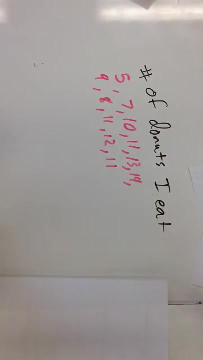 So let's say I have this data and this data is the number of donuts I eat a month. So this month kind of took it light: five donuts, but typically you can see I eat somewhere around seven to eight donuts a month. right, Not healthy, but they're delicious and I live in a town that. 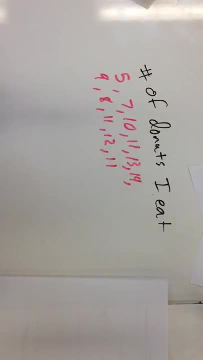 is filled with great donuts. So let's say, my brother comes into town, Joe right. So Joe comes into town and we decide: you know what, let's celebrate That month with Joe. I'm going to eat 150 donuts, Assuming that there's 30 months, 30 days in a month, we're talking about five donuts. 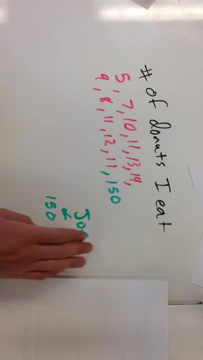 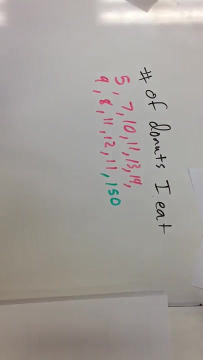 a day that I'm eating right, So when Joe's in town I kind of gorge out. So the question is: what's going to be affected Most by this? Is the median of this data going to be affected or is the mean? So the median is? 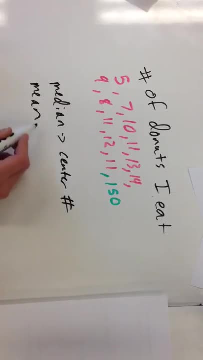 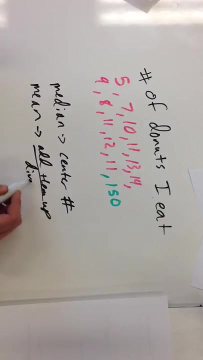 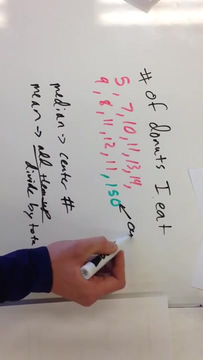 the center number, right, And the mean is we add them all up and then divide by like the total number of them, right? So what this thing right here is called? it's called an outlier, And I'm 95% sure that's how you spell outlier And mean is very. the mean is very affected by. 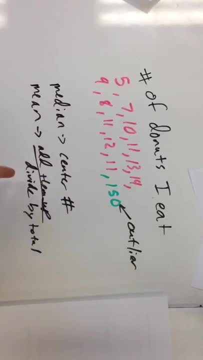 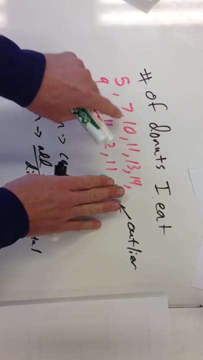 outliers because it's treated like all the other numbers. It gets added up and divided right. Try finding the mean by adding all these up and dividing by. let's see one, two, three, four, five, six, seven, eight, nine, ten, eleven. Try adding those up and dividing by eleven. Now add: 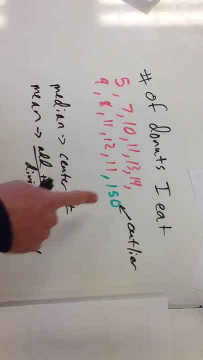 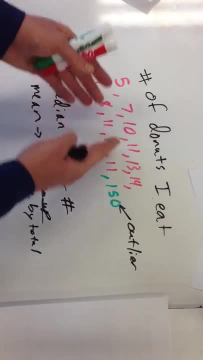 twenty fifty. fifty really affects it. The median is really good because it's outlier proof, right. So what the median says is: let's line them all up and let's cross off that gorge month with Joe. and let's cross off that month. I only ate five and let's still.